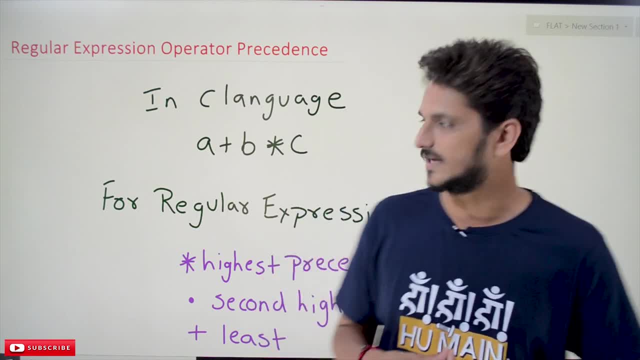 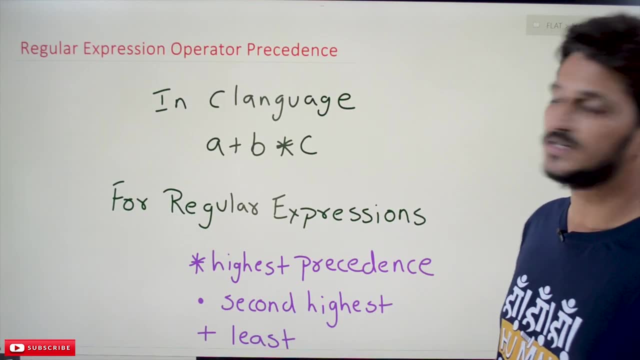 the playlist is provided in the description below. Coming to today's class, you know C language. we are having expressions, and expressions are evaluated based on precedence: a plus b, star c. So b multiplied by c will be evaluated first. The output which we got from: 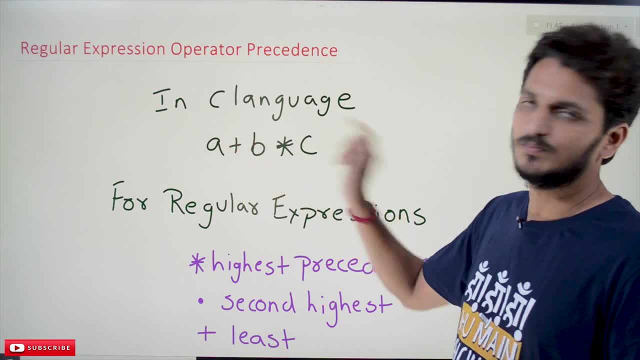 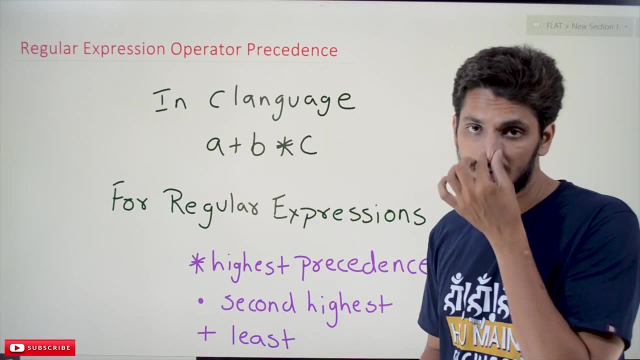 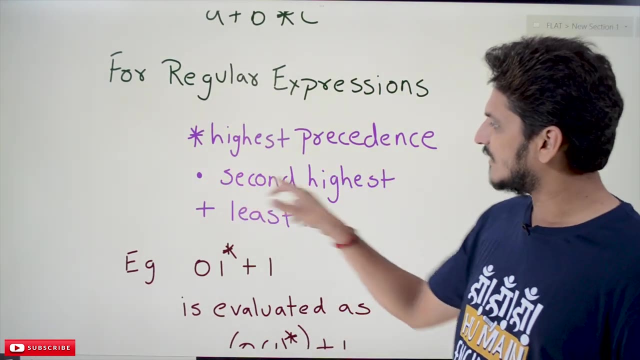 b multiplied by c is given as input to the a plus. a plus is a summation with a. This is how the expression is evaluated, because star is having the highest precedence, The same way you know regular expressions also. star is having the highest precedence, dot is having the second. 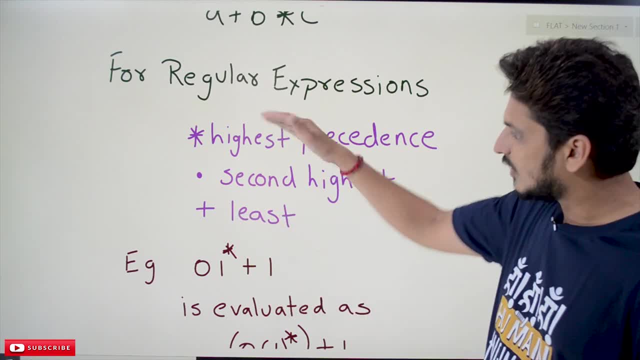 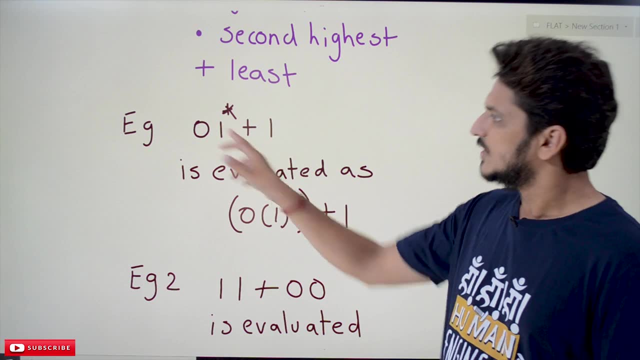 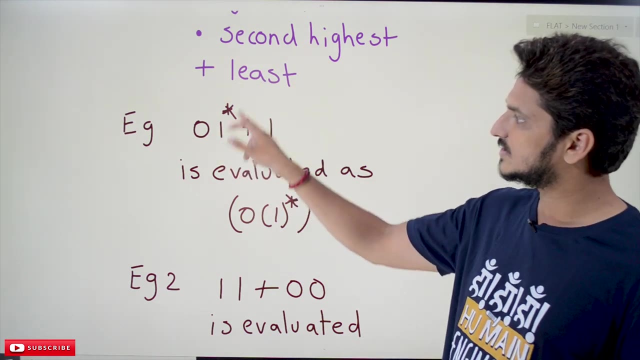 highest precedence, plus is having the least precedence. According to the precedence the expression is evaluated. Coming to an example, let's take few examples and understand: 0, 1 star plus 1. Here we are having dot operator plus operator and star operator. 0, 1 star means in: 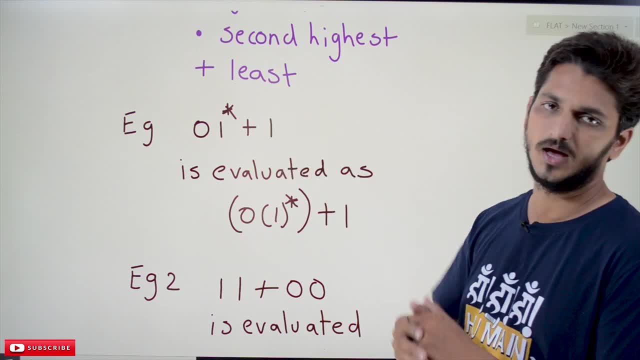 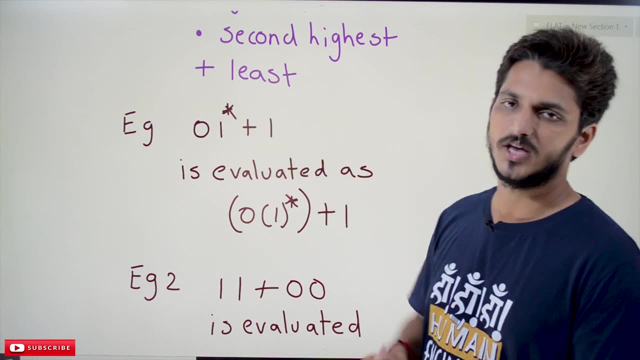 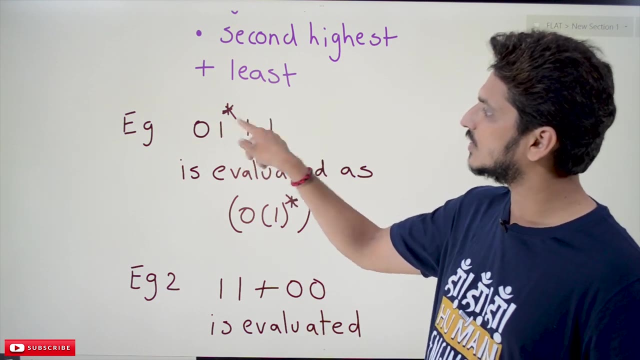 between there is a dot 0 followed by 1 star plus 1.. So out of this, which one having the highest precedence Star is having the highest precedence. That's why 1 star is taken. After taking star operator, we are having two options: 1 star plus 1 can be taken or 0 dot 1 star can be taken. 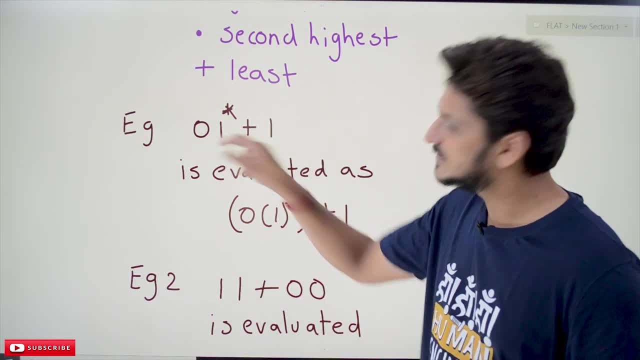 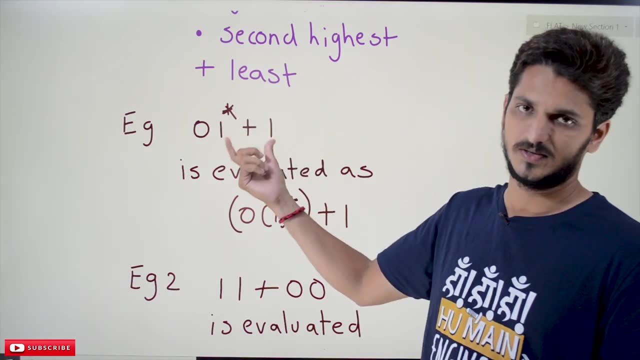 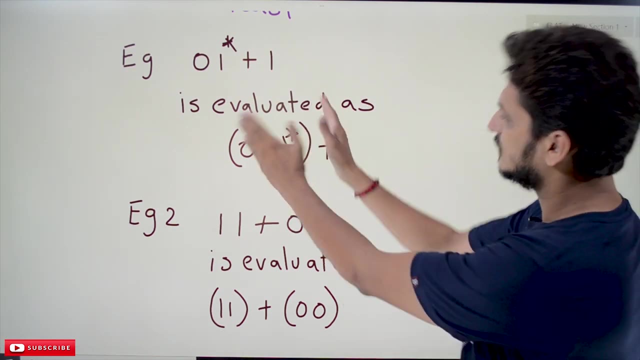 Out of this, which one is having the highest precedence? Dot is having the highest precedence. That's why 0 dot, 1 star, or 1.. This is what the expression says. This is how it is getting evaluated: 0 dot, 1 star. This is written like this: 0, 1 star, brackets, or 1.. This is how expression. 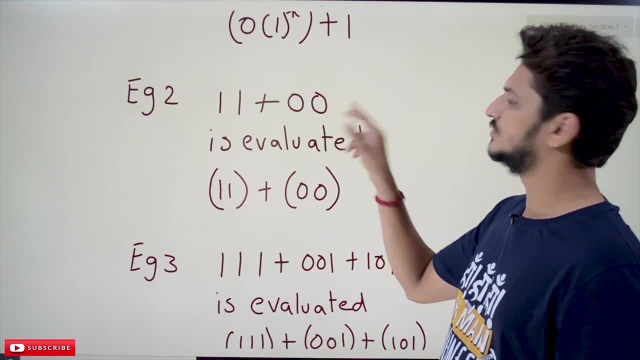 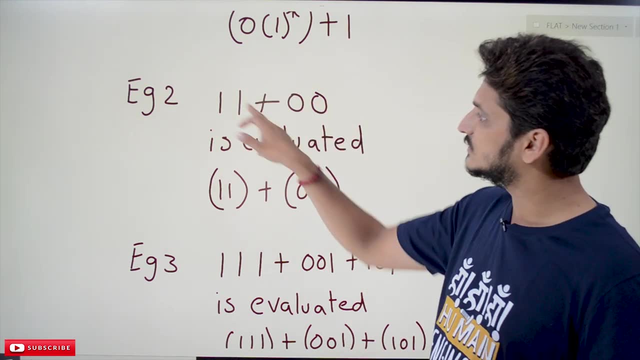 is evaluated. For example, 1: 1 plus 0- 0. Here we are having dot and plus 1 dot 1 plus 0 dot 0. Dot is having the highest precedence. That's why 1 dot 1 is taken first, 0 dot 0 is taken next, Then in between. 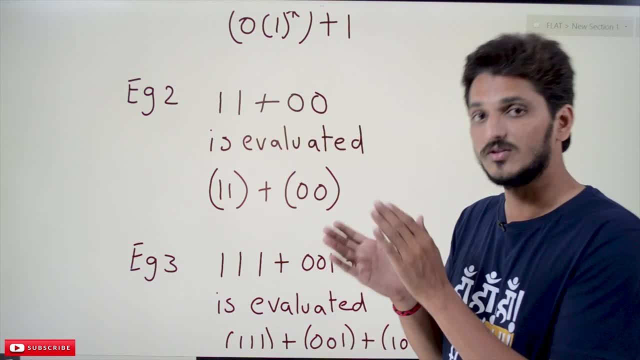 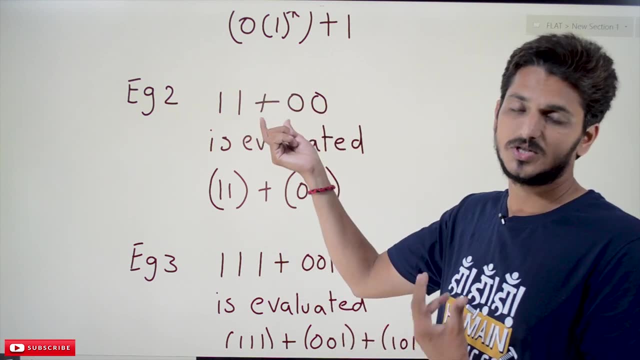 these two, we are having plus operator. That's why the expression is either 1: 1 or 0: 0.. That is what plus says: 1: 1 or 0: 0.. This expression is going to accept strings that contain either 1: 1.